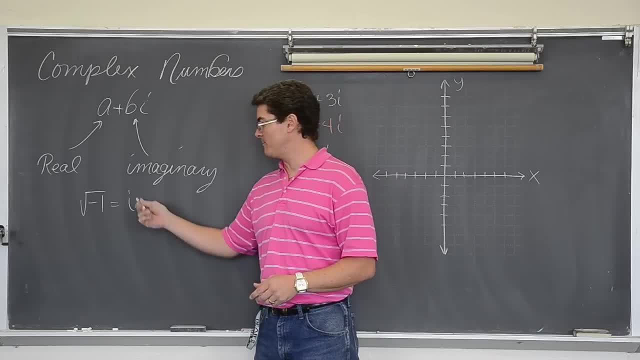 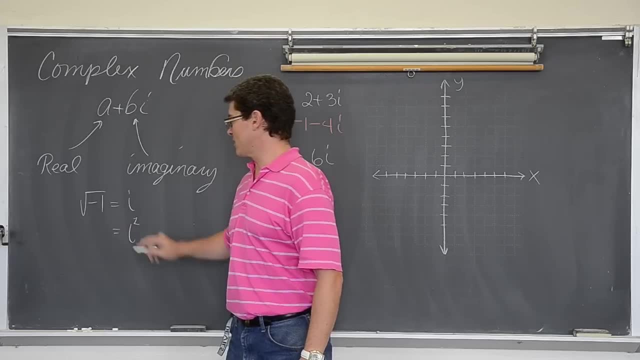 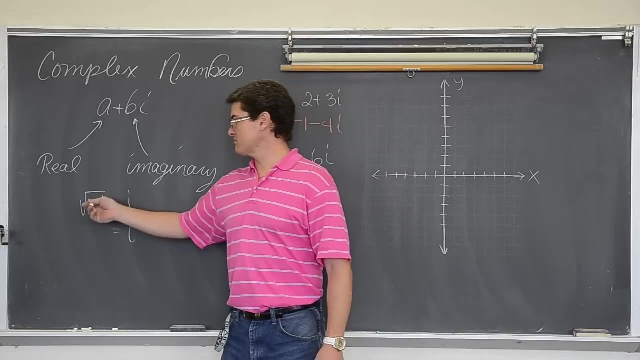 of a negative number. So we must give it this imaginary identity of i. Well, one fact that we are going to use quite a bit today is: i squared, Now i squared. I squared is well, just as it says: i times one. 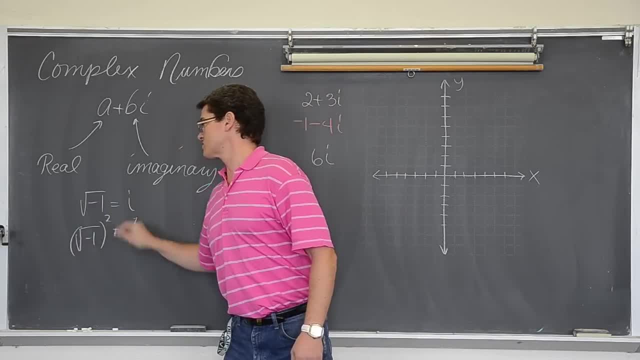 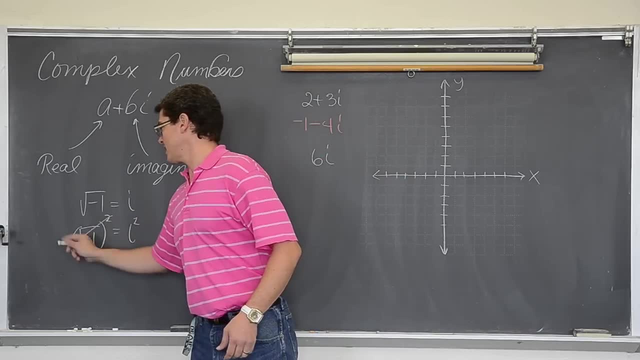 That is i or the square root of negative one squared. Well, what happens when you square a square root? Don't they cancel out? Yes, they do. So those are going to cancel out and we get that i squared is equal to negative one. So i is the square root of negative one. 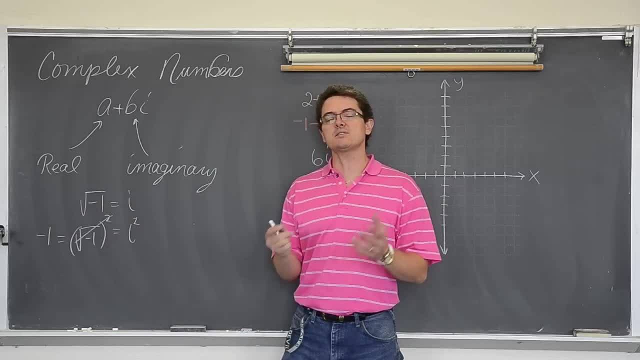 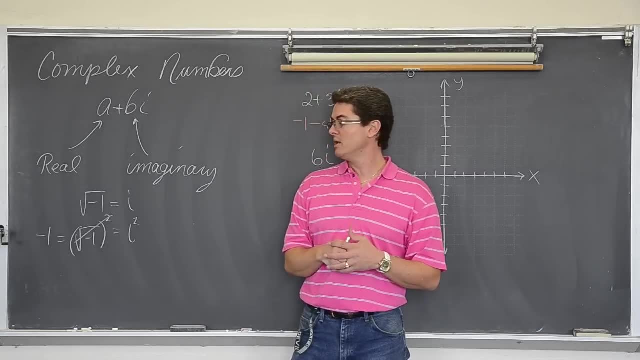 But then i squared is negative one. This is how we can use these imaginary numbers in math calculations, because, as we manipulate them more and more, sometimes we are able to cancel out that square root root that we have there and actually get a real number back that we can use in a later. 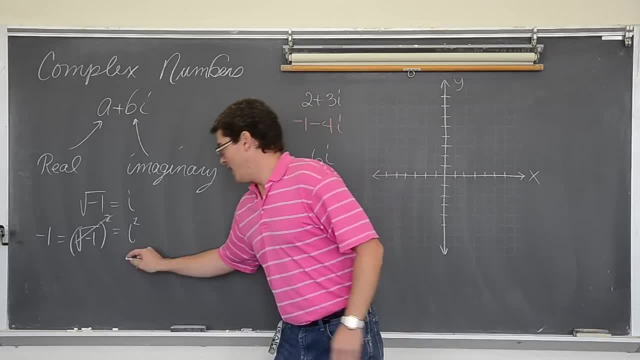 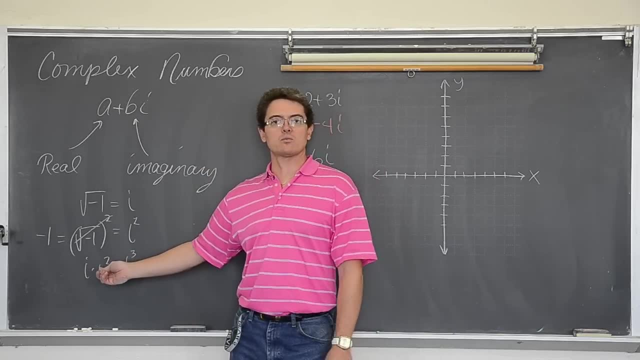 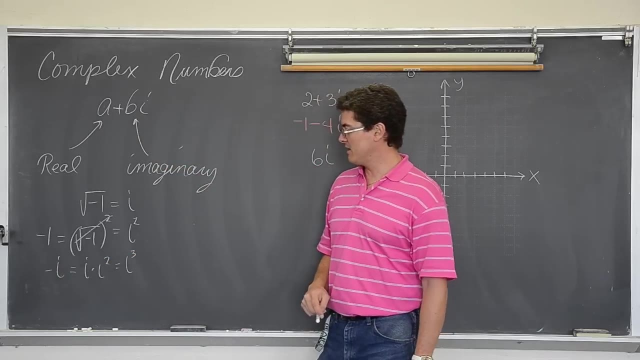 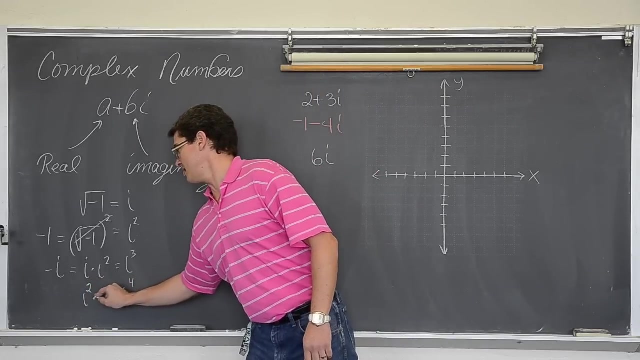 calculation. Ok, i to the third: is i times i squared? We just said i squared was what i squared was negative one. So i to the third is negative i and then i to the fourth is: well, that is i squared, times i squared which is negative, one times negative, one which is: 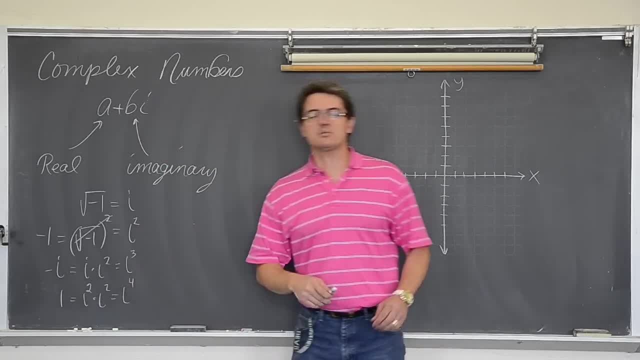 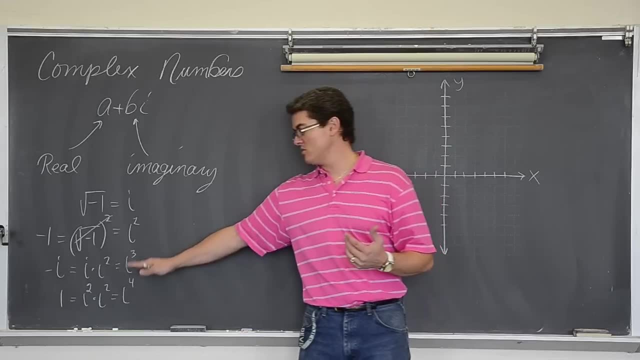 positive one. Now I am giving you these four values or powers of i, because in your book you might be using those for some questions. Now I am not going to use the third and fourth power for what I am about to run through for my students in pre-calc. This also applies. 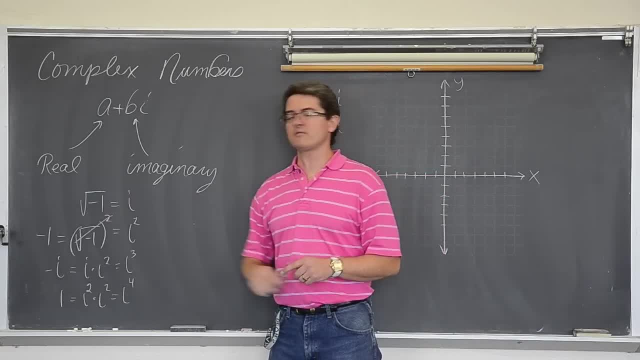 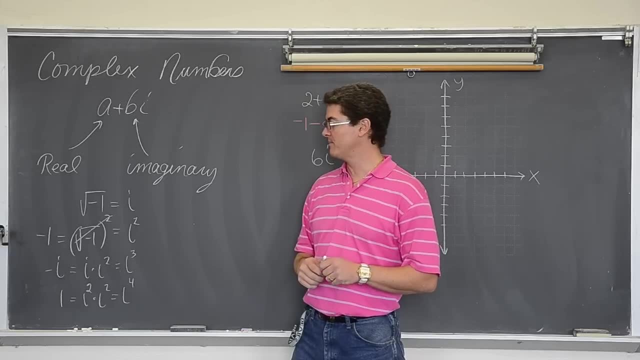 to an Algebra 2 class. I am going to be focusing on that. i is the square root of negative one, and i squared then becomes i squared Now. what is this? This is the square root of negative one. We are not doing this in. 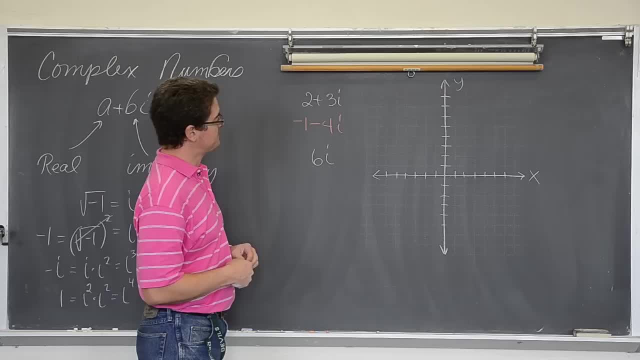 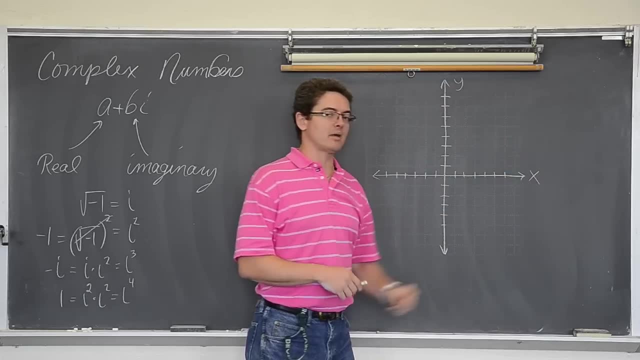 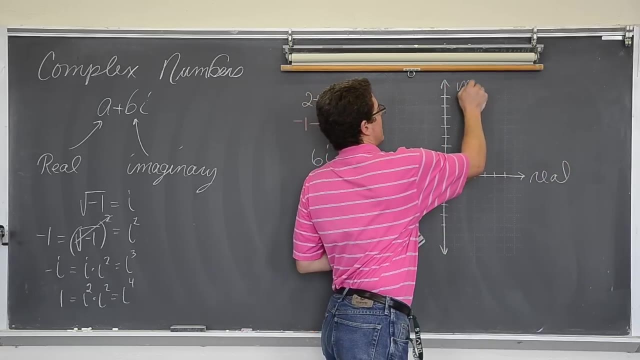 my math class. but in case you are, if you are trying to graph or draw where these imaginary numbers are on the xy axis, Well, we don't really have an xy axis when we are talking about imaginary numbers. No, we have a real axis and an imaginary axis. Now you notice. 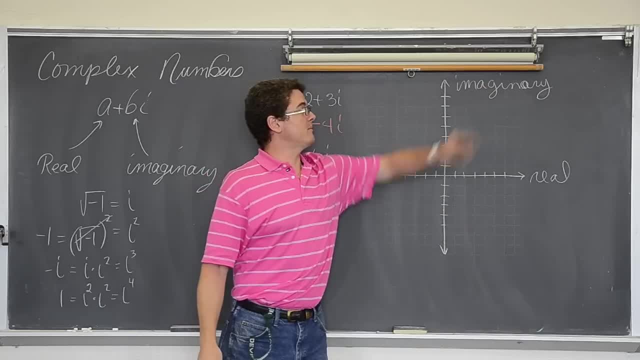 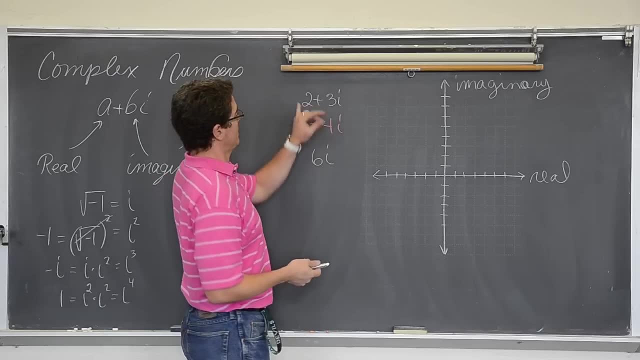 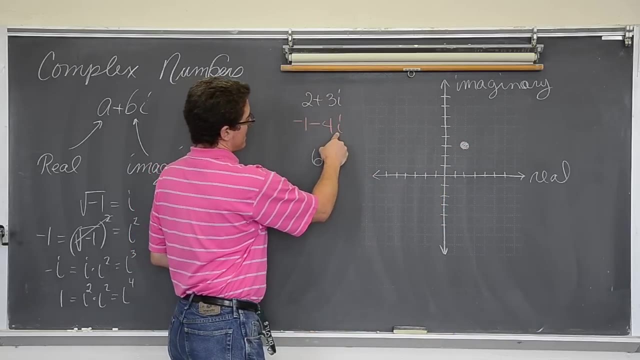 I took out the x and put in real, which is first. I took out the y and put in imaginary, which is the second number. So when you go to graph these it is going to seem like you are graphing a regular point. 2, 3i is over 2 and up, 3.. Negative 1 minus 4i is left and 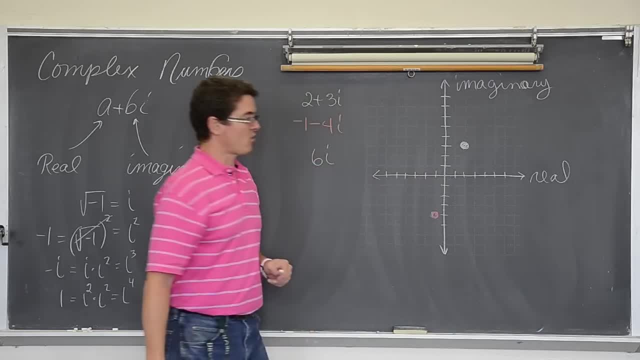 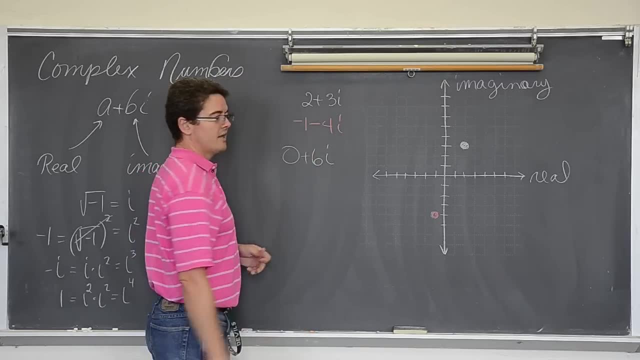 down. So negative 1 minus 4i is there. This is just 6i. Well, where is the real part Right there? No left right movement, Just go up 6.. 1, 2, 3, 4, 5, 6.. So there is a super quick. 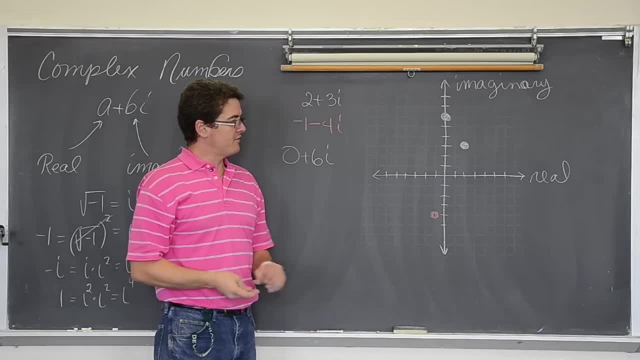 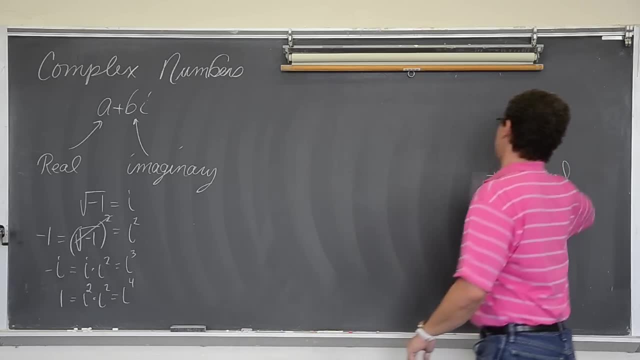 example of how you can draw or graph these three imaginary values. Now let's get into what my kids are doing, which is just some basic algebraic manipulation. Manipulation is just a basic algebraic manipulation. Manipulation is just some basic algebraic manipulation. 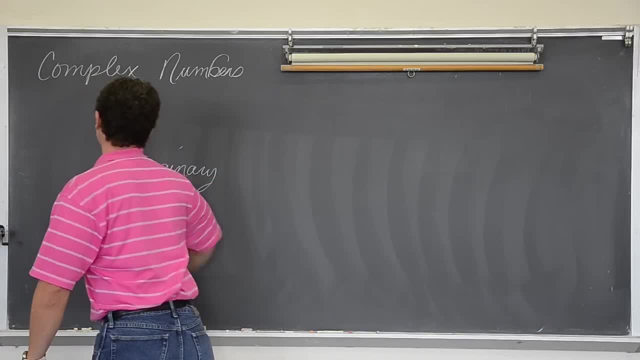 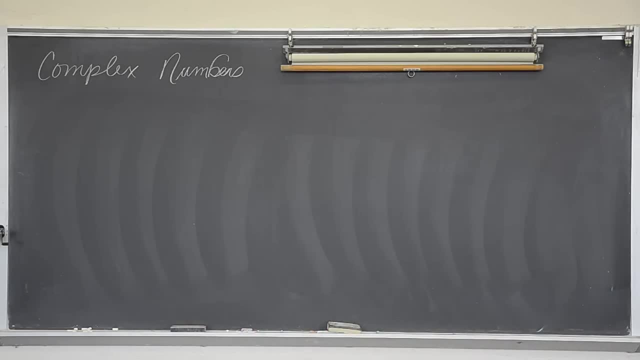 Manipulation is just some basic algebraic manipulation. Manipulation is just some basic algebraic manipulation, Manipulations that involve the value of i. Ok, let me make sure I have some time left. Ok, let's run through. I am going to go through this as quickly as I can because I want to. 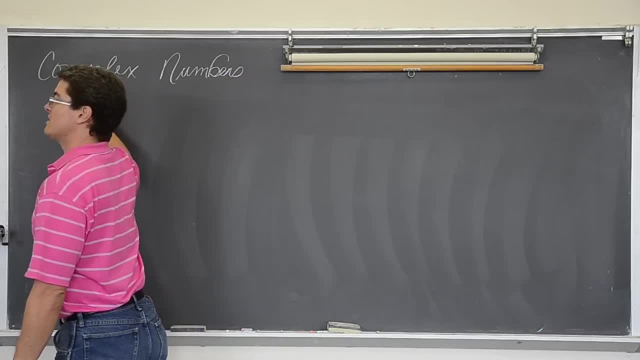 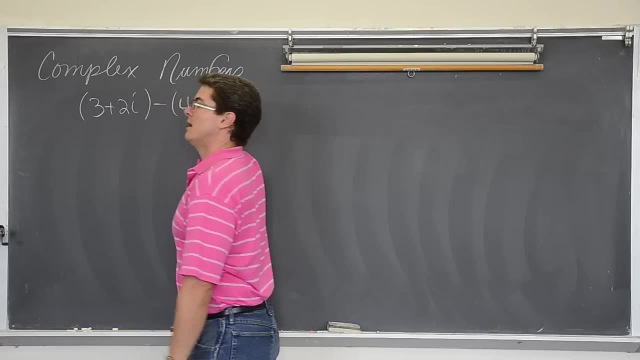 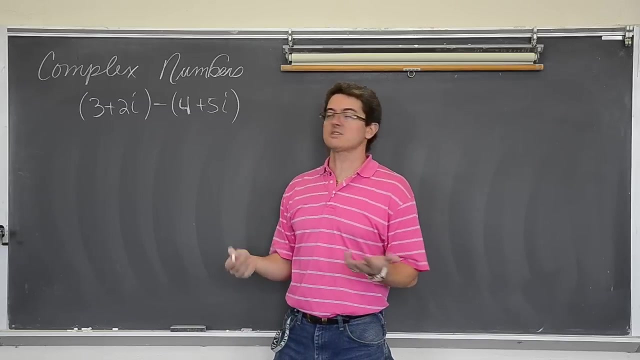 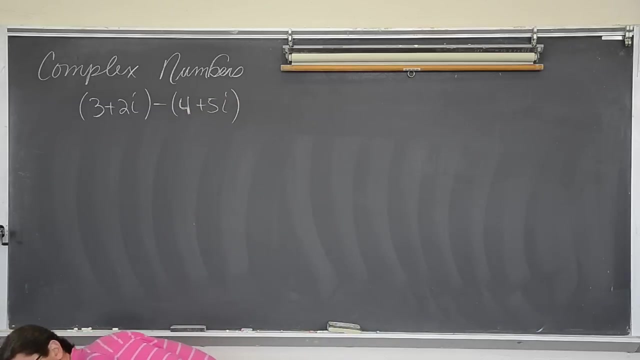 get a lot of examples done in the next 10 minutes. We have got 3 plus 2i minus 4 plus. Well, I am just giving you some binomials, two complex numbers, and asked you to basically simplify. You are going to do this just like you deal with your generic little combining like terms. 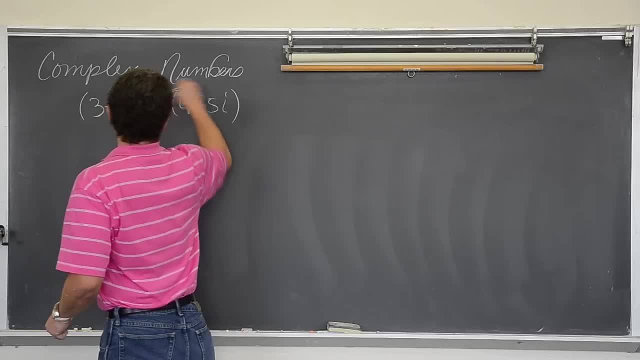 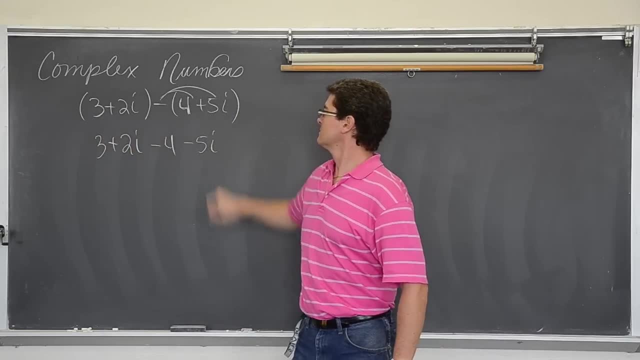 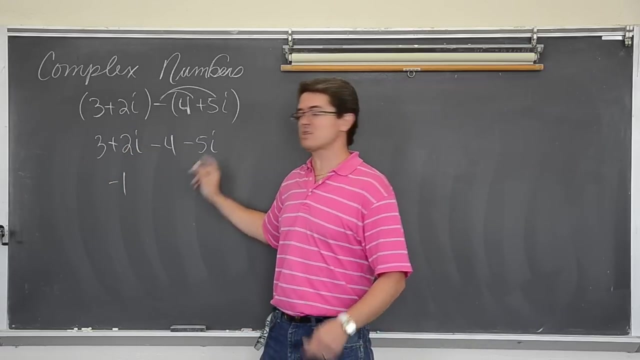 and getting rid of parenthesis. things Distribute to get the negative through the parenthesis And look for like terms 3 and negative 4. Negative: 1.. What about 2 and negative 5?? Well, 2 minus 5 is negative 3i. 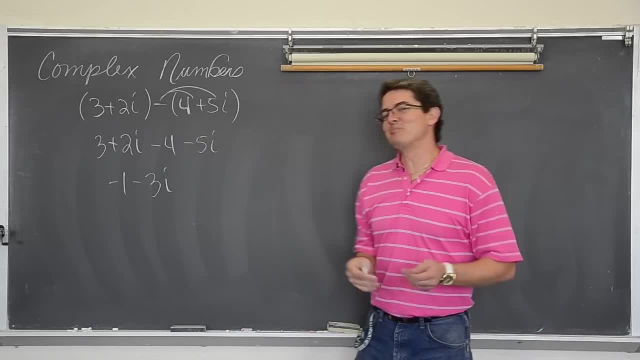 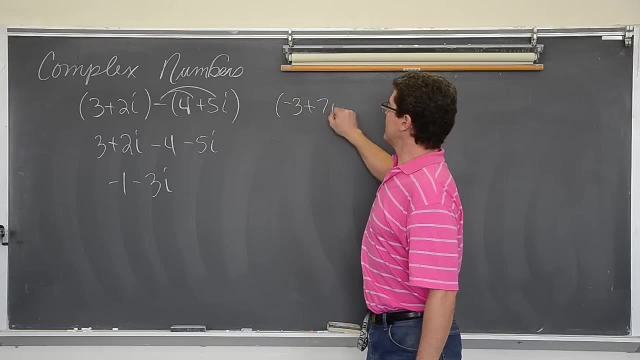 Real and imaginary. So it looks very similar to basic algebra skills you have done for a long time. Let's take a look at this example: Negative 3 plus 7i squared. Oh, How many times do I see kids mess this up? 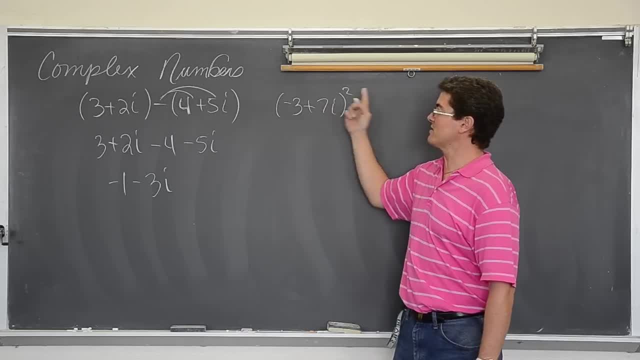 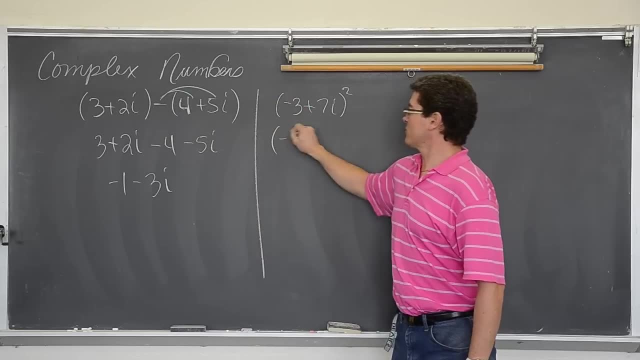 We have a binomial squared. It's not 3 squared and 7 squared. No, no, no, no, It's negative. 3 plus 7i squared Is negative. 3 plus 7i times negative, 3 plus 7i. 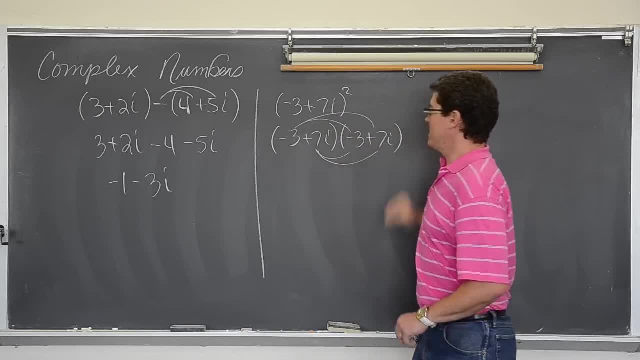 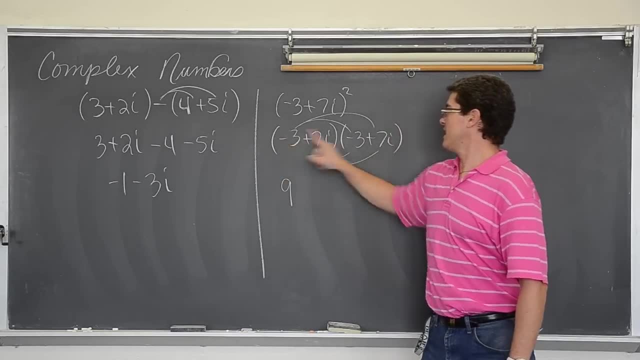 Please take the time and save your teacher a lot of grief and actually distribute those together, please, so that you have all the terms. You don't miss one. Negative 3 and negative 3 is 9.. Negative 3 and positive 7 is negative 21.. 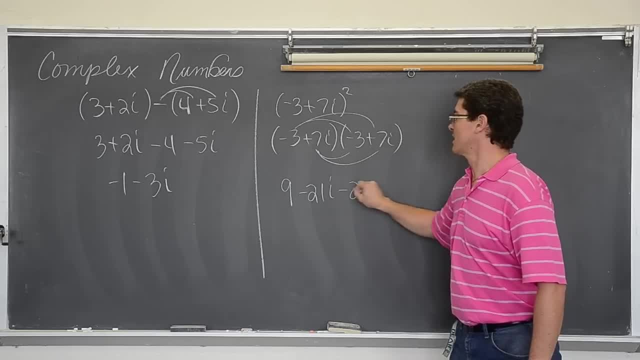 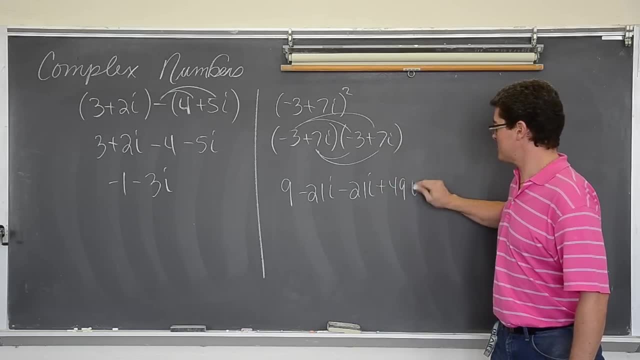 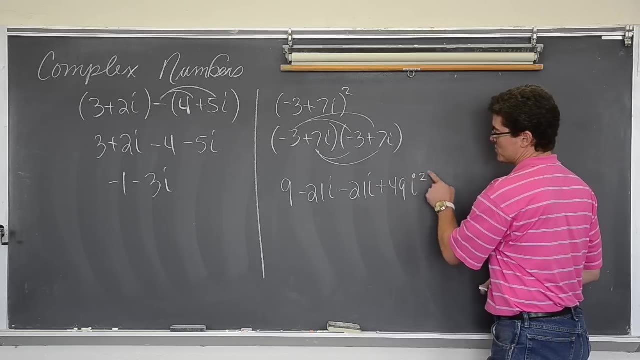 And going to the next set of lines: negative 21, again i, And then positive 49.. Oh, Negative 49i squared, And here we start. this is the only place where there is a difference when you are working with complex numbers compared to just your regular algebra. 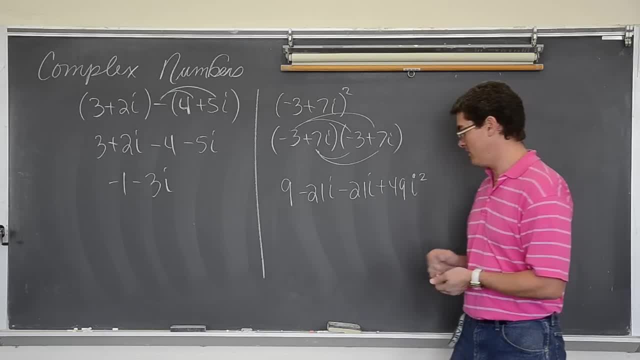 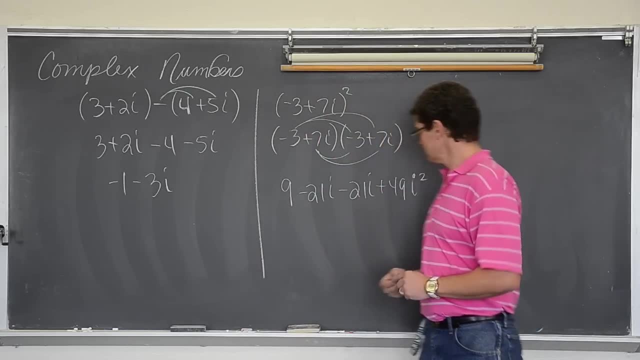 Instead of this just being like an x squared, it's i squared. Well, we just talked about- oops, I erased it. We just talked about how i squared was equal to negative 1.. So this i squared comes out to be negative 1.. 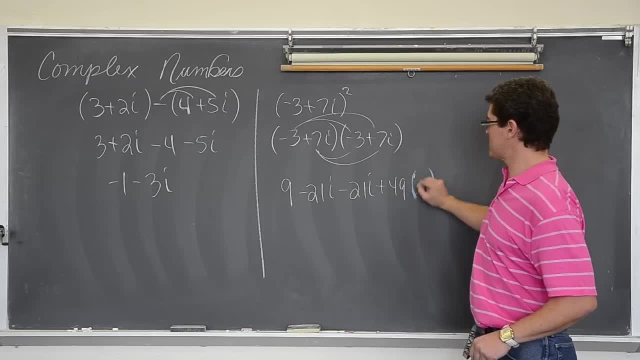 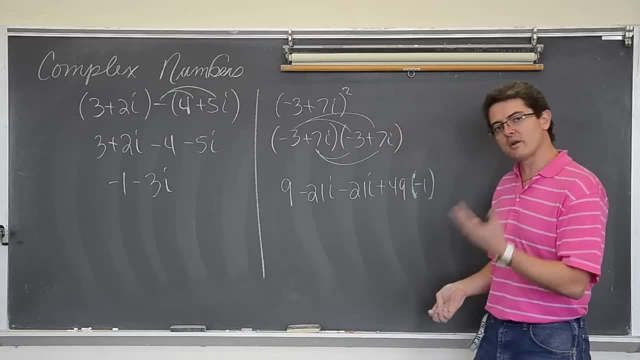 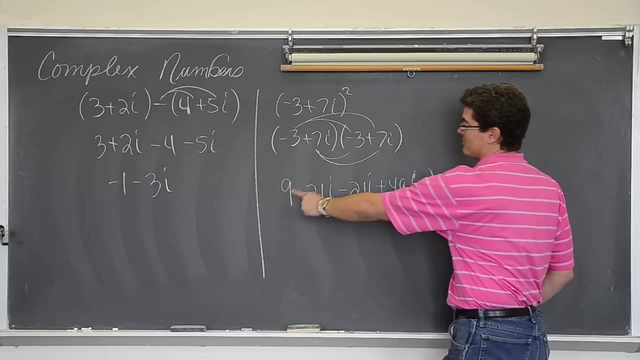 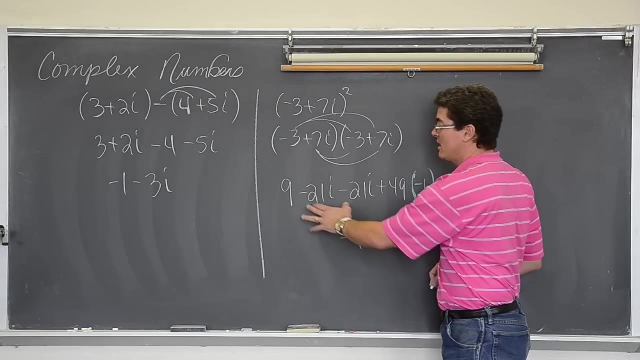 And now we are going to combine like terms. We have 9 and this is going to be negative 49, so negative 49 plus 9 is negative 40. And we have two like terms with our i's. Now they are not i squared, so the i's are going to stay there. 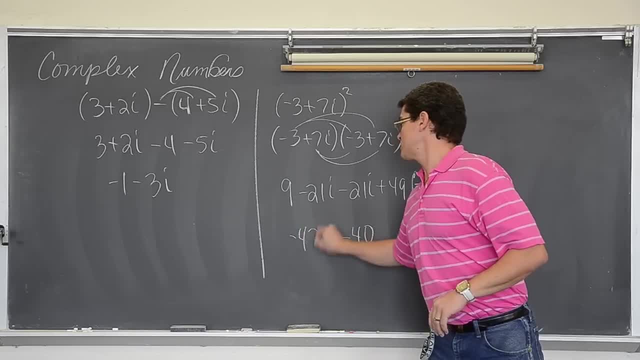 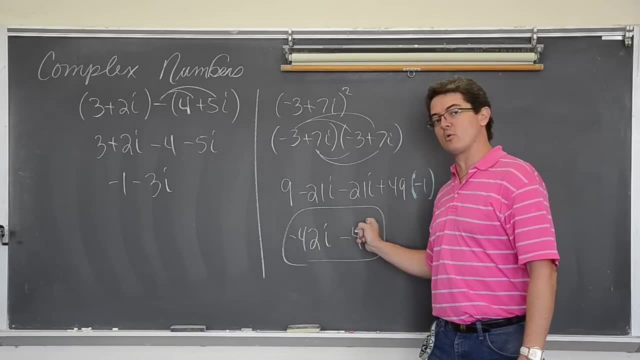 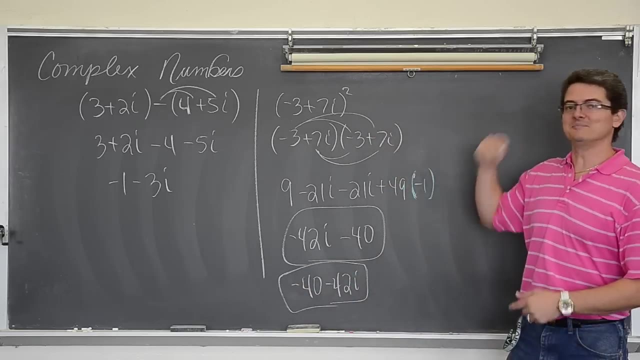 Negative 21, and negative 21 is negative 42i. Now for proper form. I need to write this in the other way, because the last one is going. real should come before the imaginary. So negative 40 minus 42i, BAM, Alright, moving. 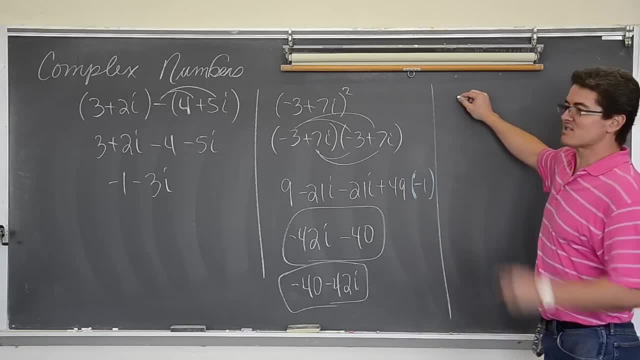 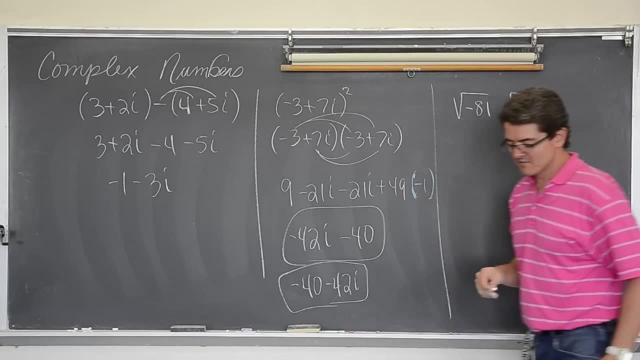 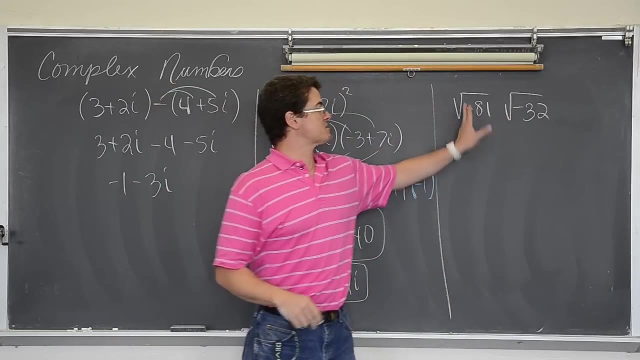 on. Did I wake you up? Let's take a look at this: The square root of negative 81 times the square root of negative 32.. You cannot work with radicals that have negative numbers inside of them. If you just multiply these together and get positive, whatever, I can't. 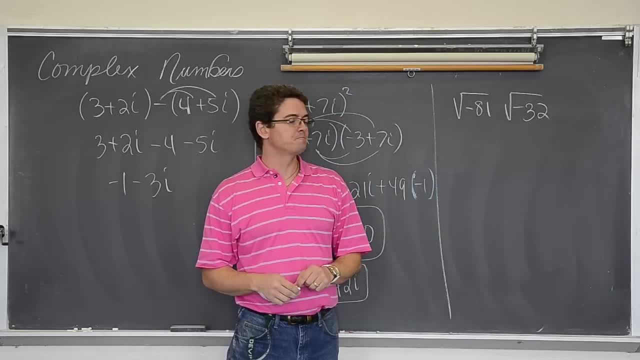 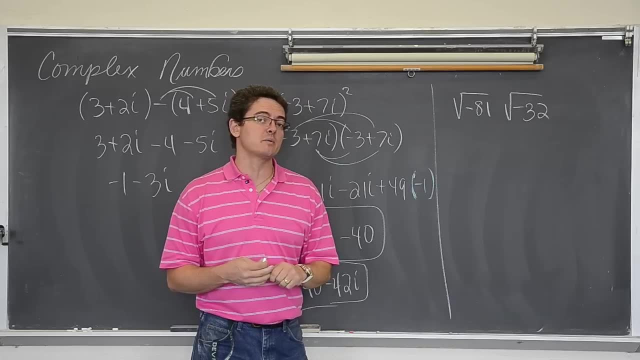 do that in my head, you are going to get a number that is much, much too big- Excuse me, not too big. You get a sign error. You believe that your answer is positive, but you will see in a minute that it is actually supposed to be negative. If you have negatives and 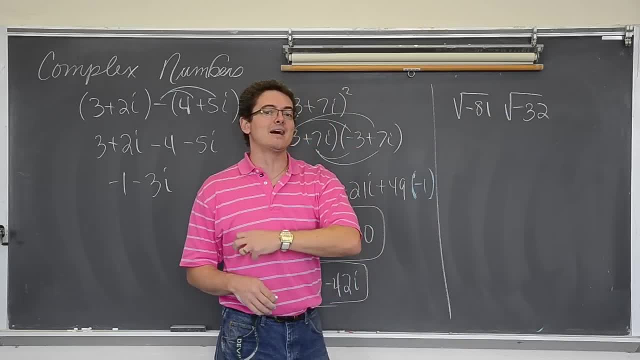 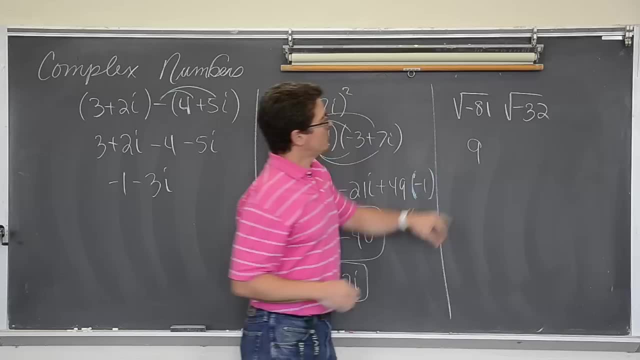 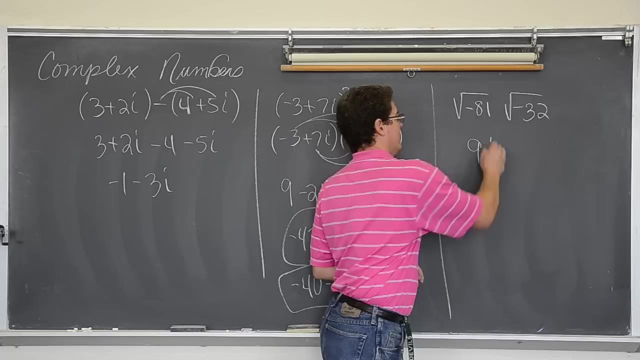 their real values inside your square root symbols. you need to pull those out, as i's before you start Now. 81, the square root of 81 is what It is: 9.. What is the square root of negative 1?? Because 81 is negative, The square root of negative 1 is, i Times. well, what is going? 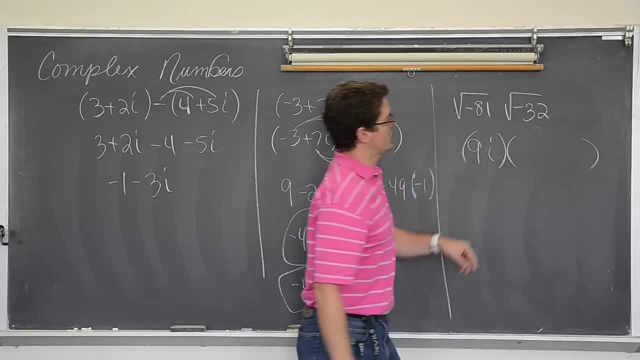 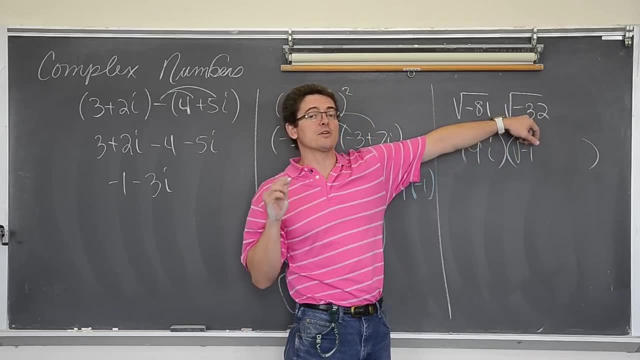 on over here. Now I am going to break this up a bit more, just to make sure you understand what I am doing. I have got negative 1, so the square root of negative 1.. And 32 won't square root, but there is a perfect square in 32.. I am going to reduce this. There is. 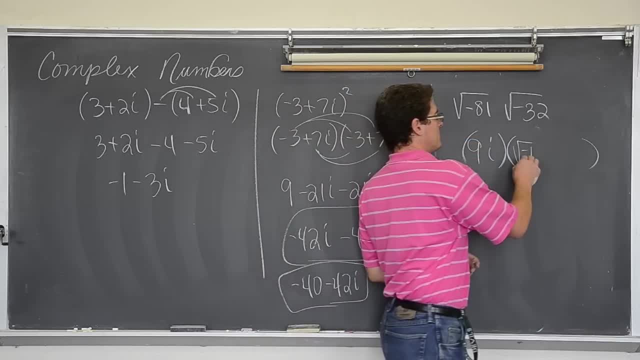 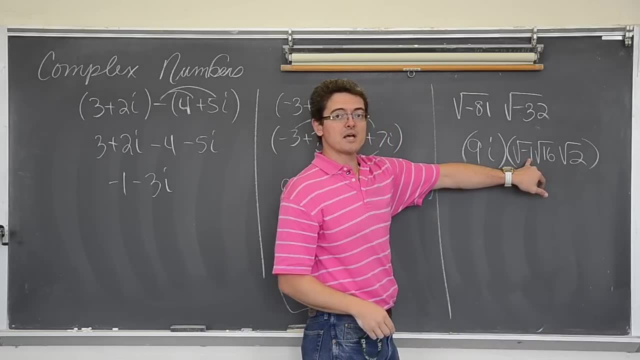 a 16 times 2.. So the negative 1, I am going to leave it separate. The square root of 16 times 2 is i and the square root of 2.. Well, the square root of negative 1 is i and the. 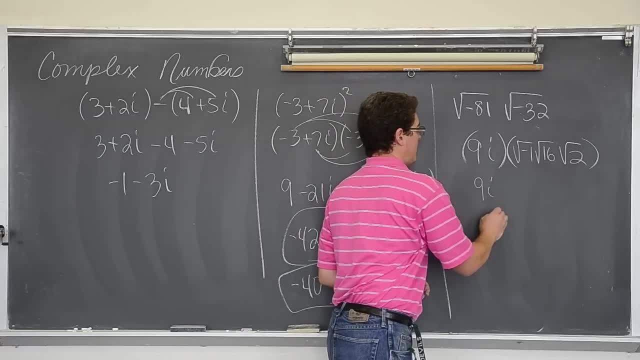 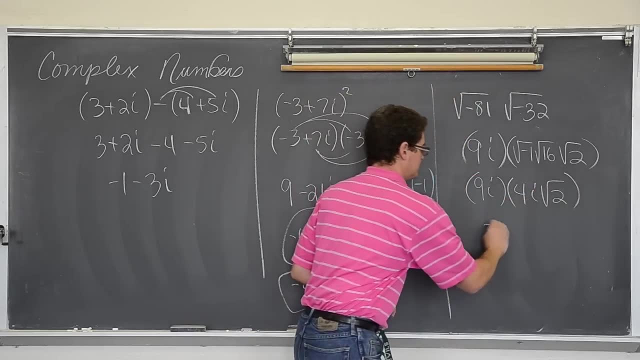 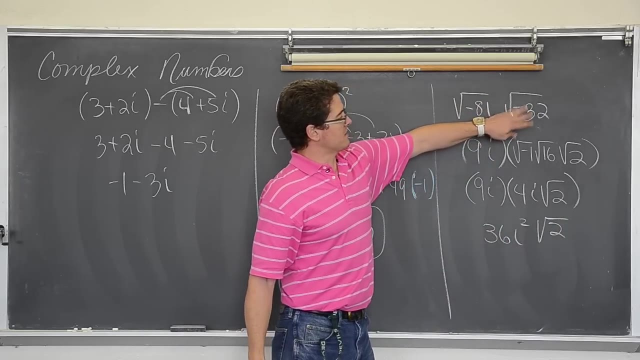 square root of 16 is 4.. So we are going to have 9i times 4i square root of 2.. 9 and 4 is 36.. i squared and 2.. Now, if I had left this the way it was and I just multiplied? 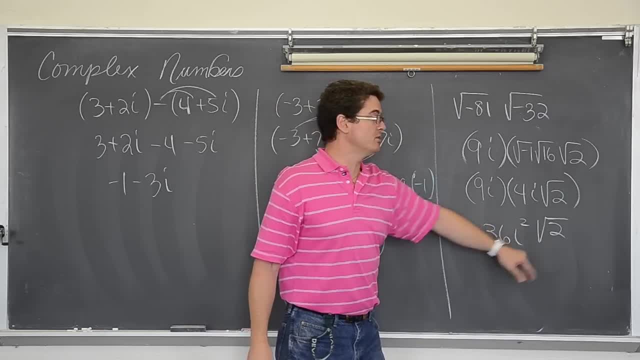 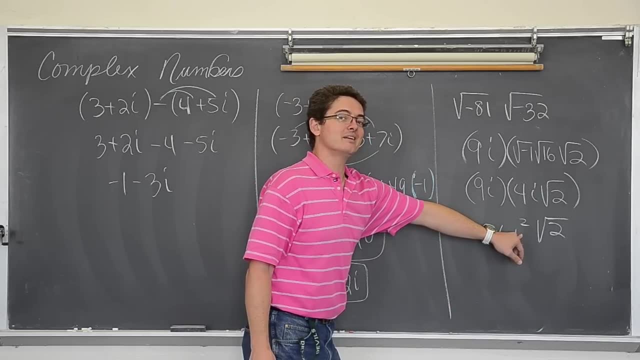 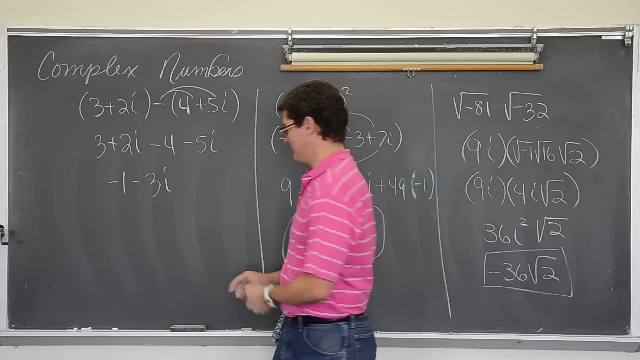 my answer would be positive: 36 square root of 2.. But if I take the i out, like I am supposed to, i squared is what? Yeah, it is negative 1.. So, negative, 36 square root of 2.. BAM, Alright. 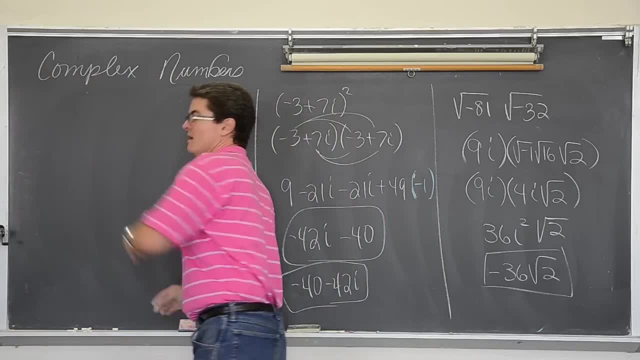 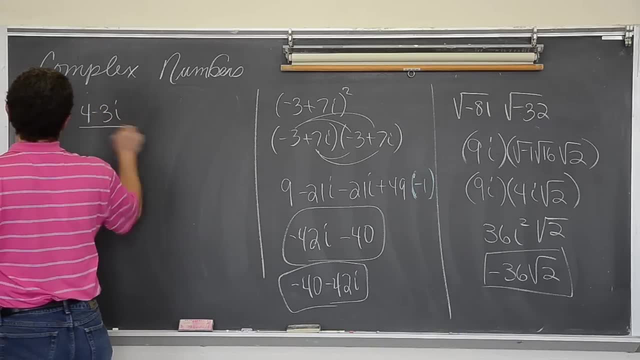 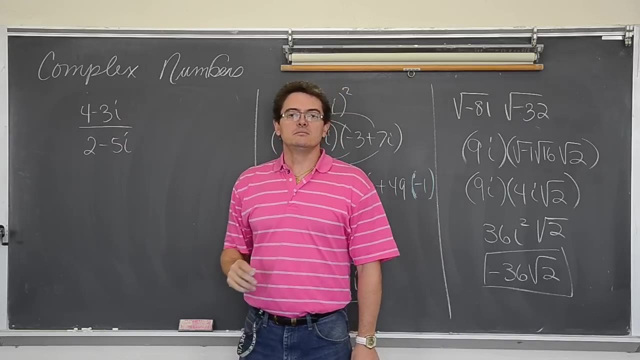 Let's take a look at another example. Let's take a look at 4 minus 3i over 2 minus 5i. Simplify this. Well, it looks pretty simple. I am going to take the i and the square root of 2.. It is pretty simple already. If this were an x instead of an i, it would be done. 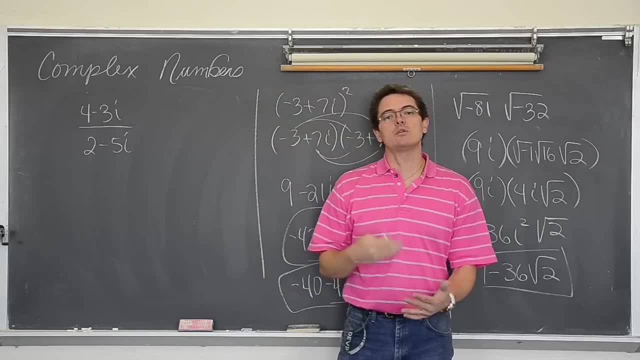 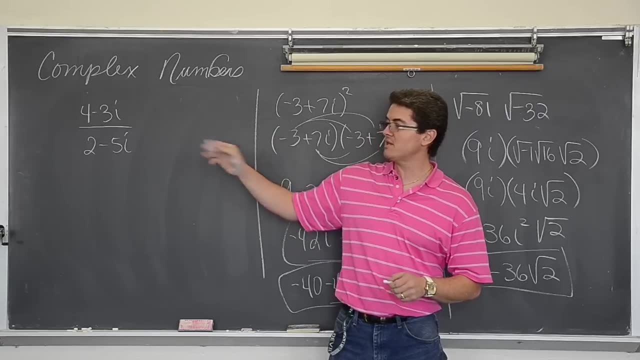 But i is a square root right. i is a square root of negative 1. And you can't leave a radical in the denominator, if you are right in your final answer. So this, though it doesn't look like it, needs to be rationalized. We need to multiply by something that will get. 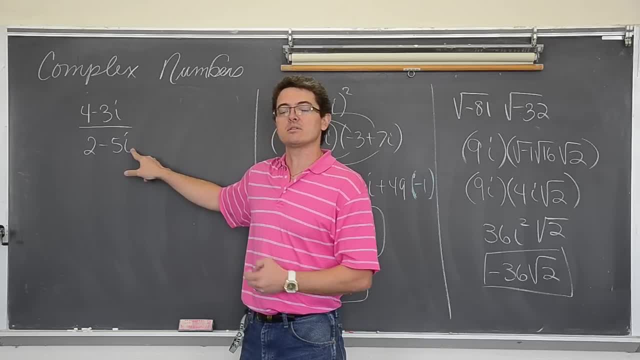 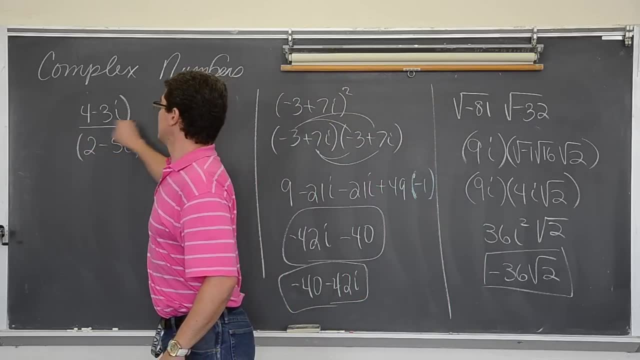 my square root of negative 1, my i out of the denominator. And you do that when you have binomials by multiplying by the square root of negative 1.. And you do that when you have a conjugate by something called the conjugate, Which means that you simply change the sign. 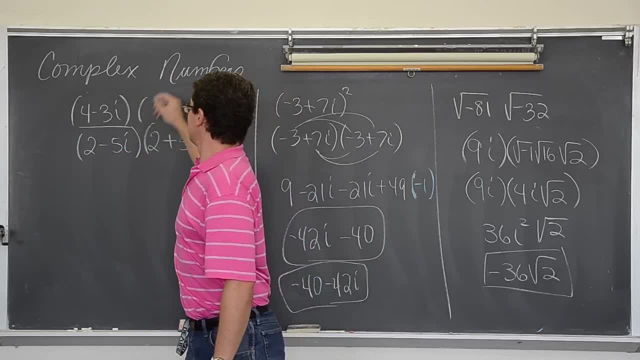 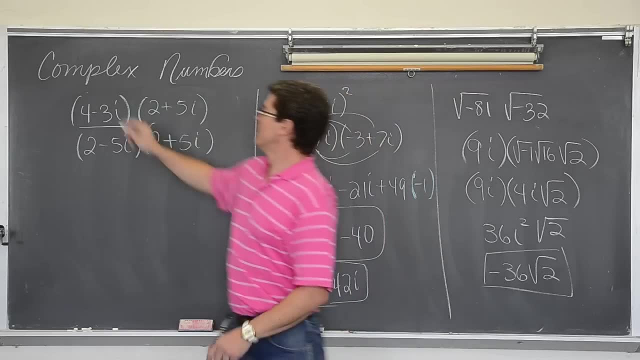 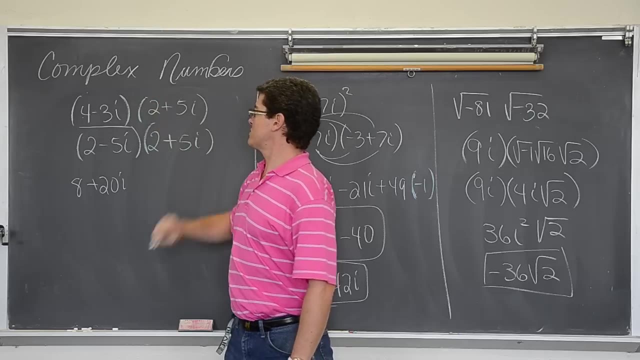 the middle sign and multiply that to the top and bottom of the fraction. So we are going to get 4 times 2 is 8,. 4 times 5 is positive 20,. negative 3 and 2 is negative 6i. negative 3 and positive 5 is negative 15i. 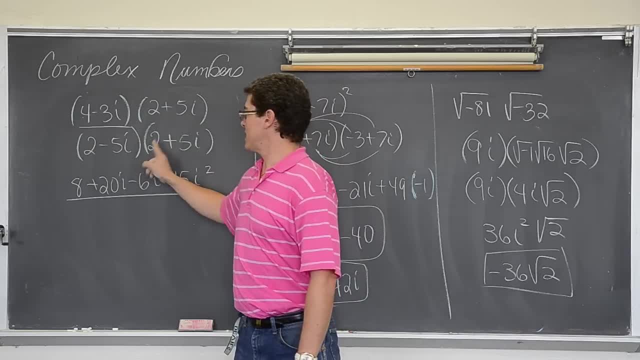 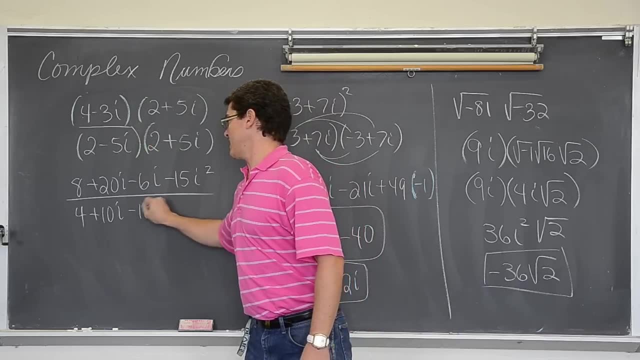 I squared all over 2 times, 2 is 4.. 2 times positive: 5 is positive, 10i, Negative 5 and 2 is negative 10i. You might not need to show this work because you know the middle term. 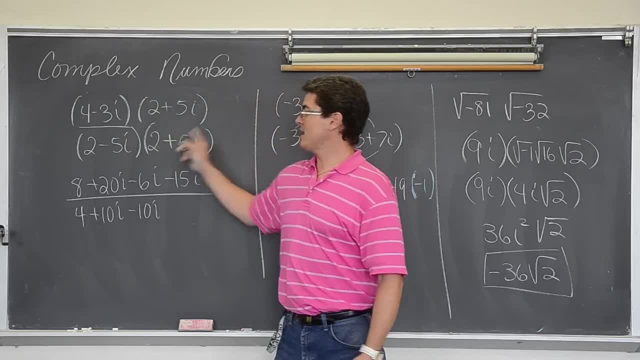 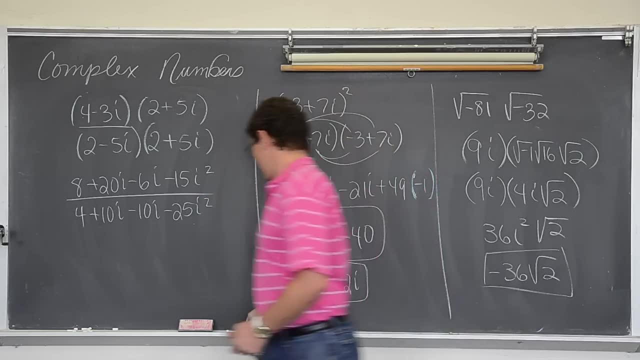 is going to cancel out, but you know I am teaching so I have to. And negative 5 and positive 5 is negative 25i squared, So we have got the positive and negative 10 canceling out And because of space I am not going to be able to do that, So I am going to do the. 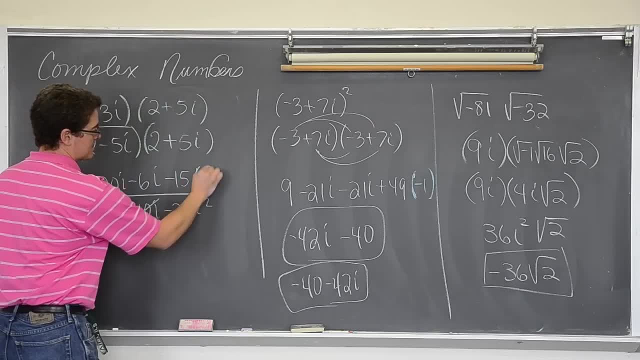 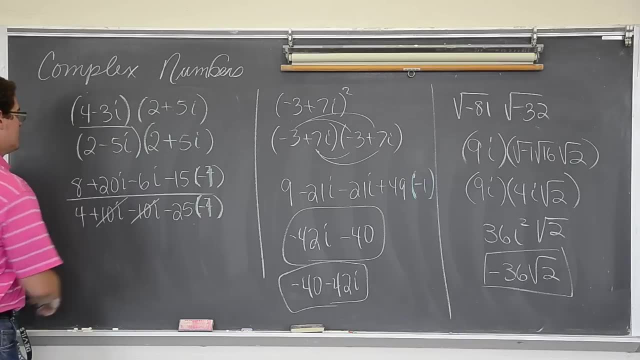 same thing over and over again. I am going to do the same thing over and over again And because of space, I am not going to write a new line. but what is i squared negative 1.. What is i squared negative 1?? So we have 8 and that is positive 15, right? So 8 and 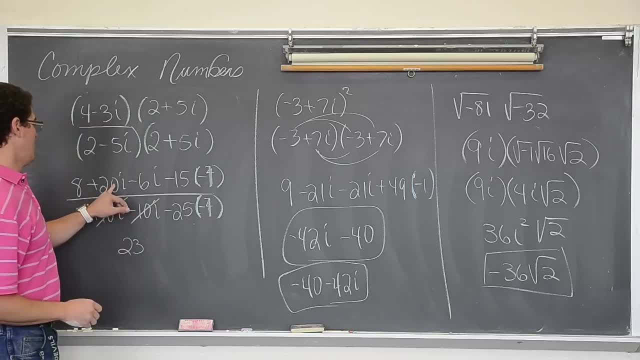 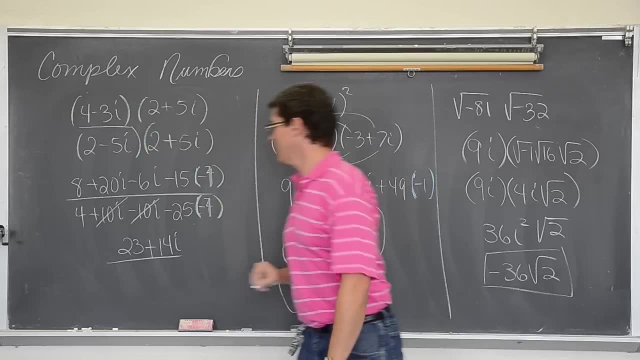 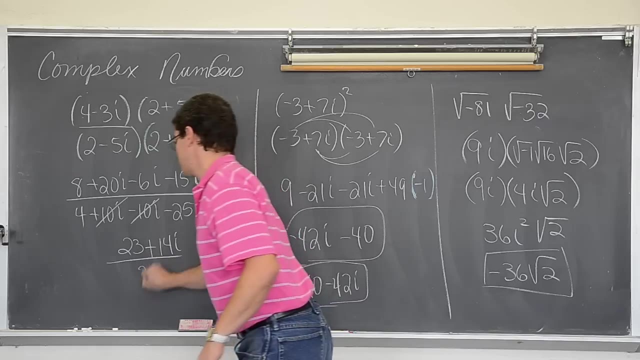 15 is equals 23.. What do we have here? We have got: 20 minus 6 is equal 14, over 4 minus So 4 and a positive 25 make 29.. Now, this is not done. Complex numbers must have a real and an imaginary part. 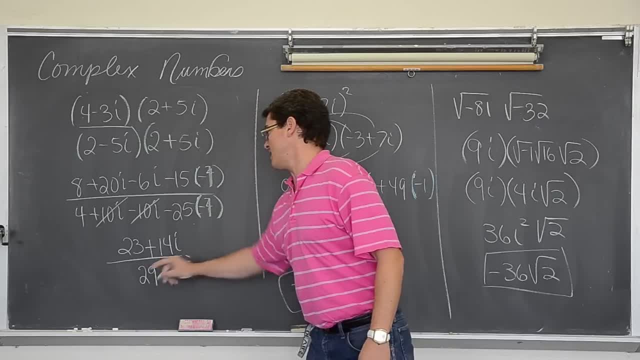 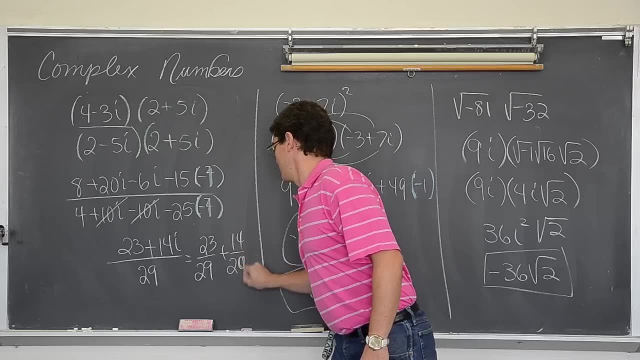 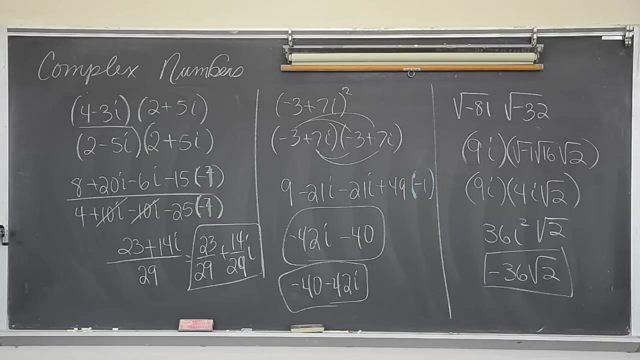 So I am simply going to split this apart and give each fraction it's own denominator of 29.. And BAM Got it done. I got two and a half minutes. Let's see if we can try and solve a quadratic formula, shall we? 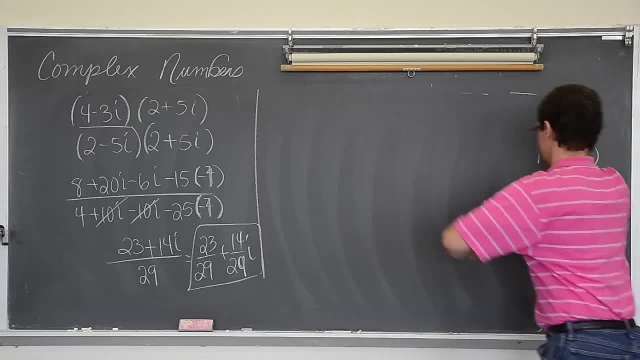 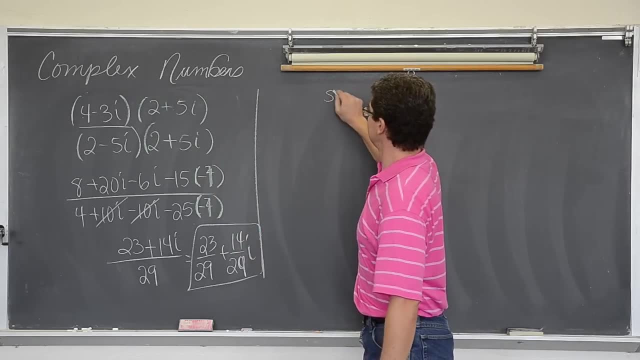 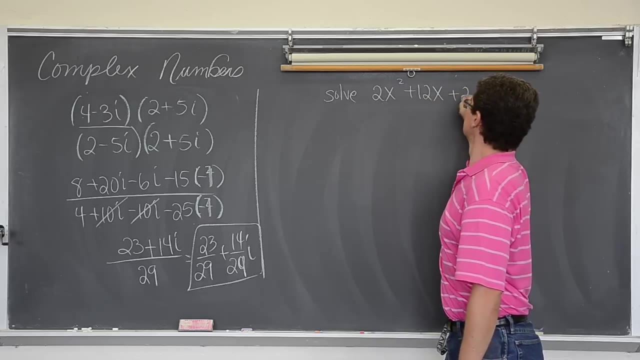 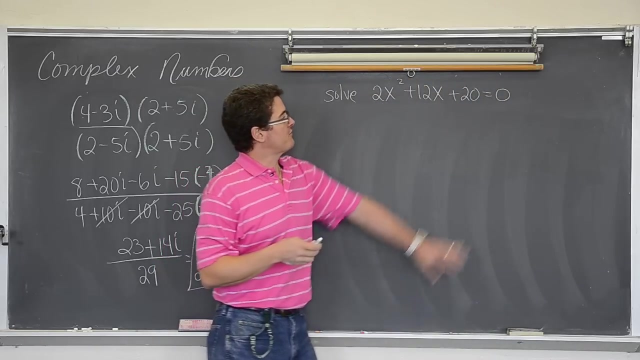 Or a quadratic equation. Ok, last example, Let's see if we can solve this equation. Now, don't forget: when you solve an equation, you are trying to find out where that equation crosses the x axis. We are trying to find out when y equals zero.